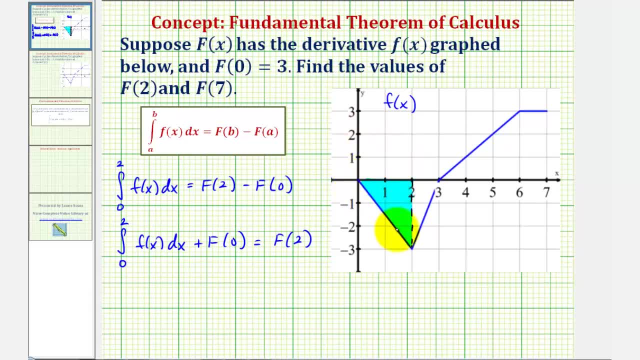 But because the area is below the x-axis or because the function values are negative, we do want to view this as a negative value. So using the area formula for a triangle, area equals 1 half base times height, We would have area equals 1 half times the base of 2 times the height of 3.. 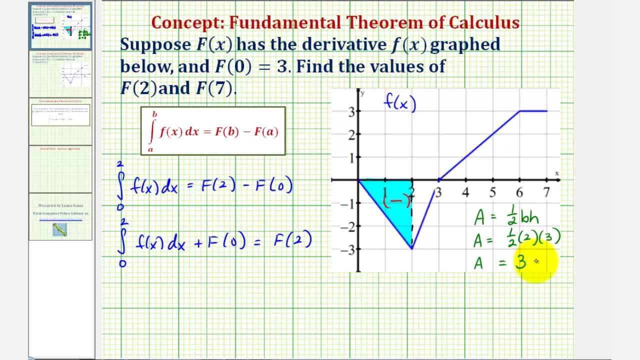 So the area of this triangle is equal to 3 square units, But because the area is below the x-axis, the value of this integral is going to be negative, 3, and then plus the value of big F of 0, which is 3.. 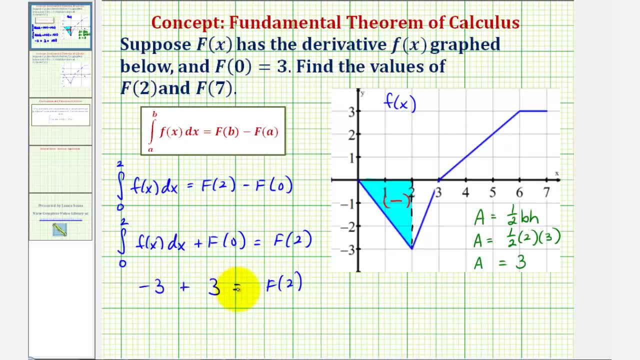 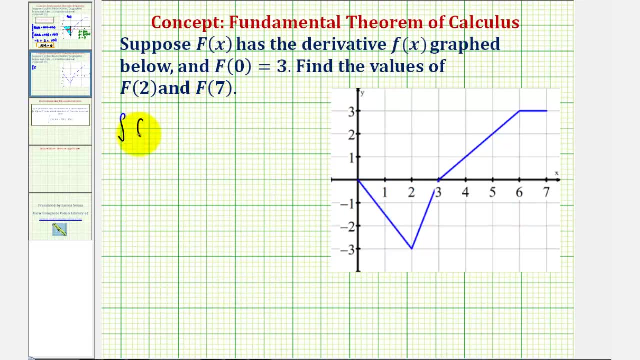 So notice that big F of 2 is equal to 0.. Now let's determine the value of big F of 7.. The def integral of little f from 0 to 7 must equal big F of 7 minus big F of 0.. 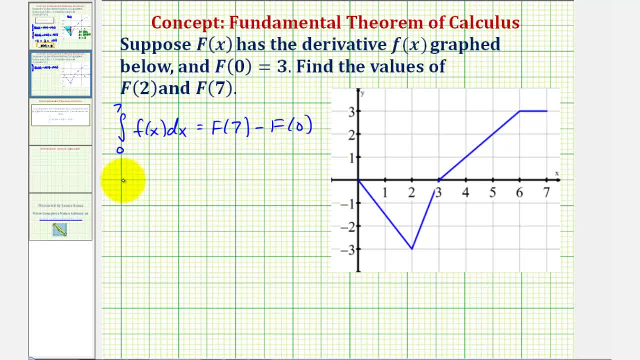 So all this, or big F of 7, will add big F of 0 to both sides, giving us the integral of little f from 0 to 7 plus big F of 0 equals big F of 7.. Now we'll work on determining the value of this def integral. 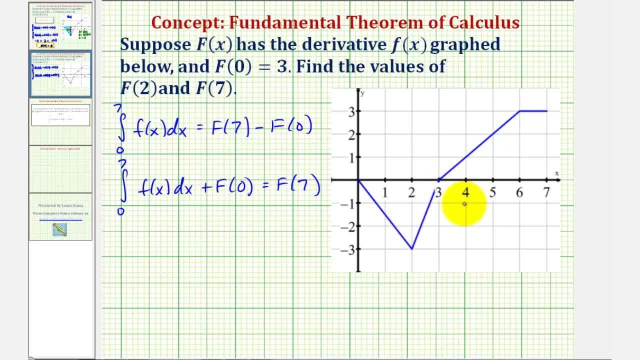 by analyzing the graph of our function f of x here on the side. Let's first shade the area bounded by the function on the x-axis over the closed interval from 0 to 7.. And again, because this area is below the x-axis for the value of the def integral, we need to view this as a negative value. 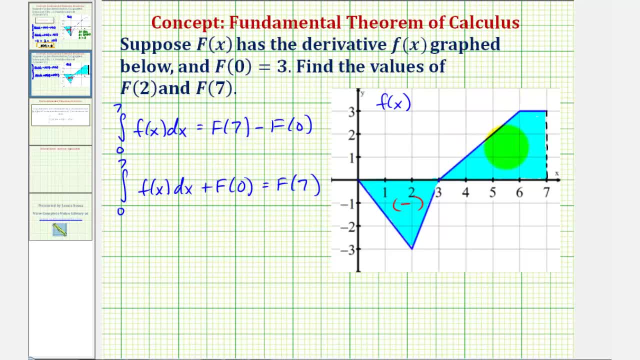 And because this area is above the x-axis, we can think of this as a positive value. Let's go ahead and call this a sub 1.. Let's divide this here. Call this a sub 2 and a sub 3.. So the area of a sub 1 is going to be equal to. 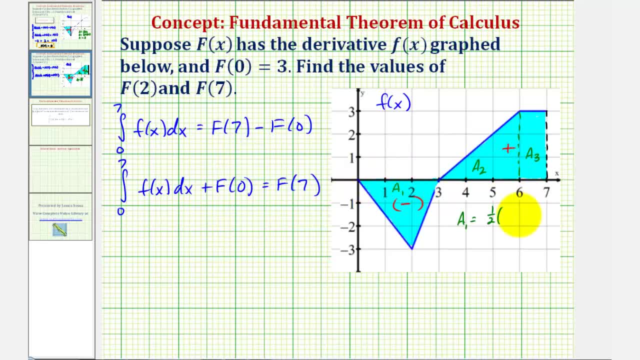 1 half times the base of 3 times a height of 3.. So that's equal to 9 halves, even though for the def integral it would be a negative value. And now for a sub 2, this right triangle, here the area is going to be equal to 1 half times.